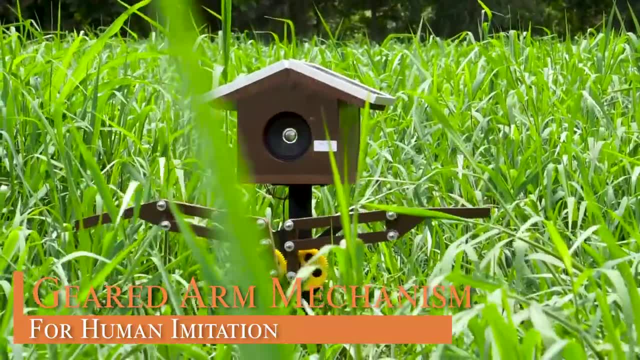 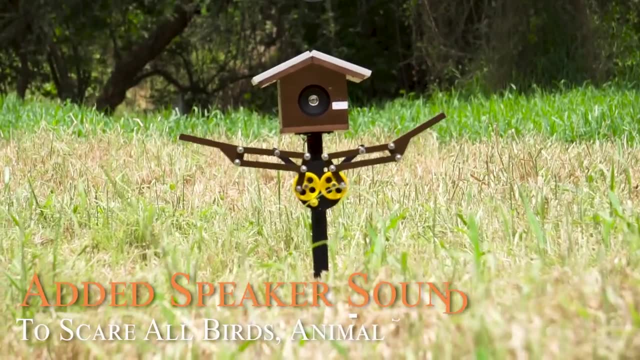 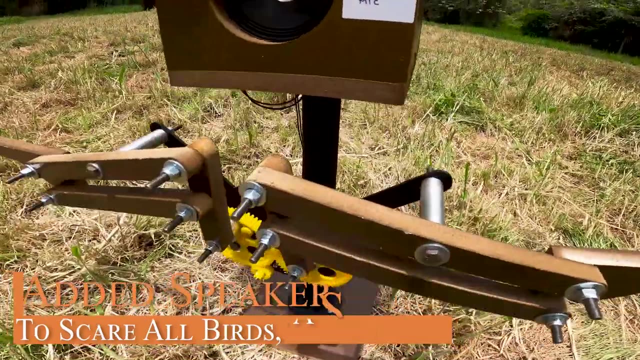 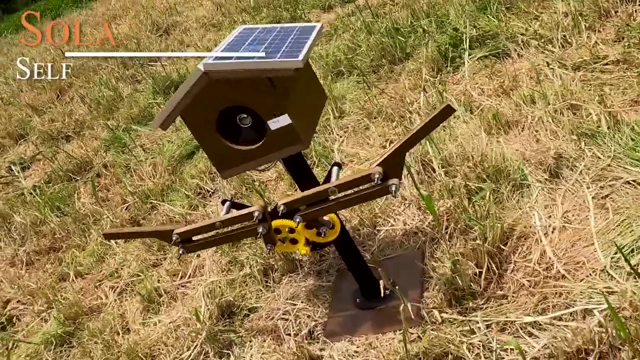 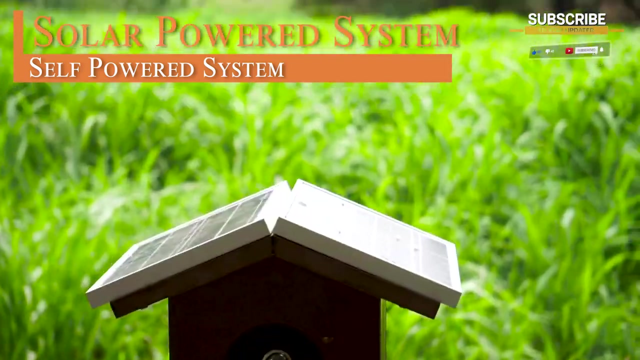 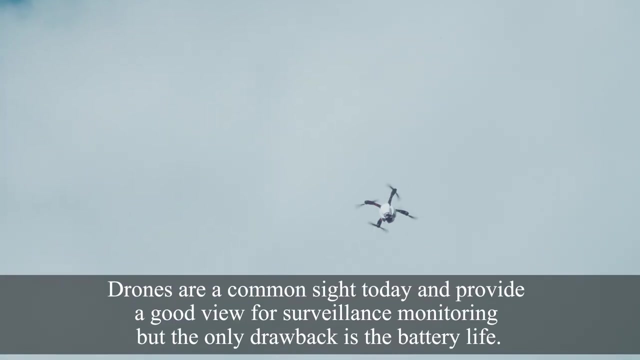 Now, without any external power. the Scarecrow is ready to take off. It is ready to be in the sun. Self-Charging Surveillance Drone Drones are a common sight today and provide a good view of surveillance monitoring, but the only drawback is the battery life. 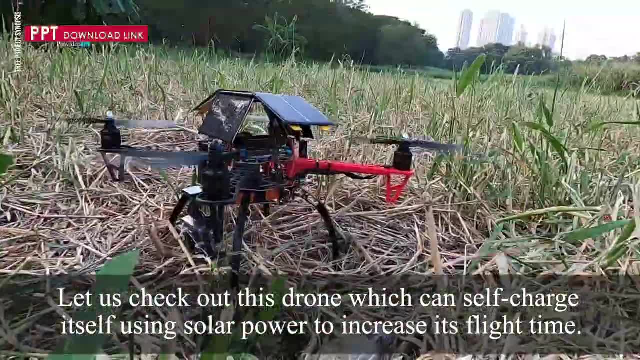 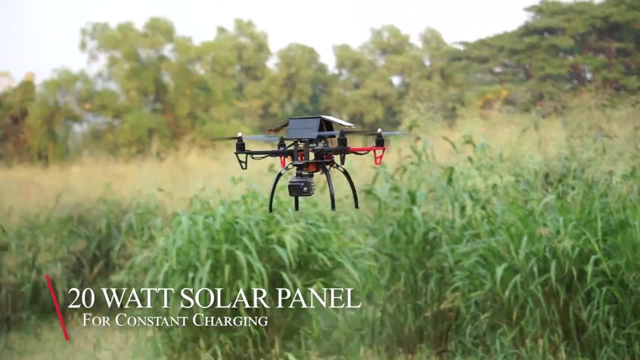 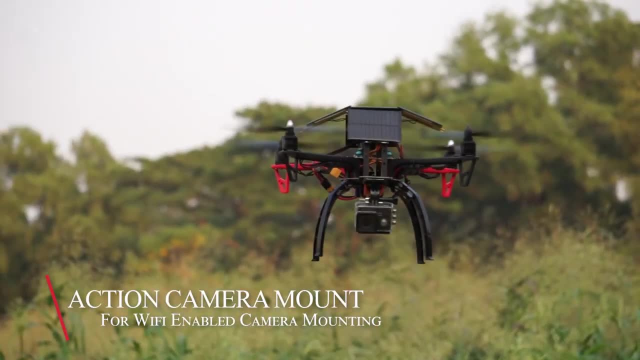 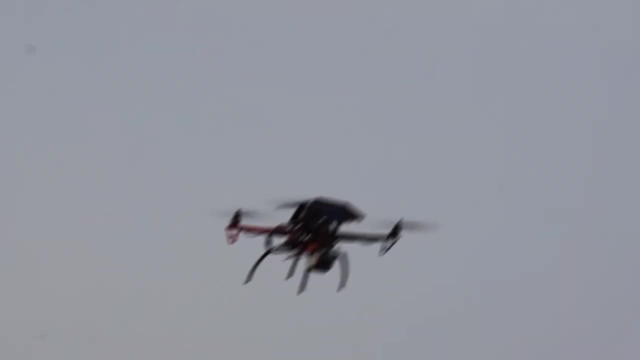 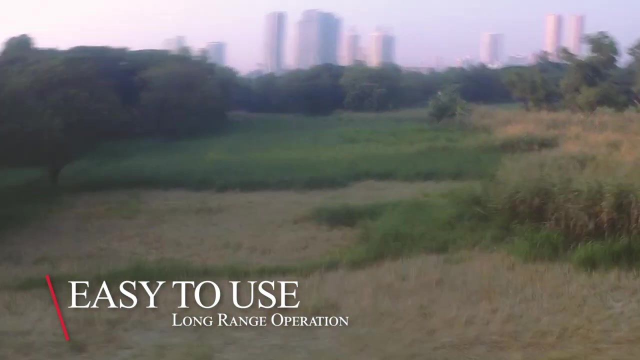 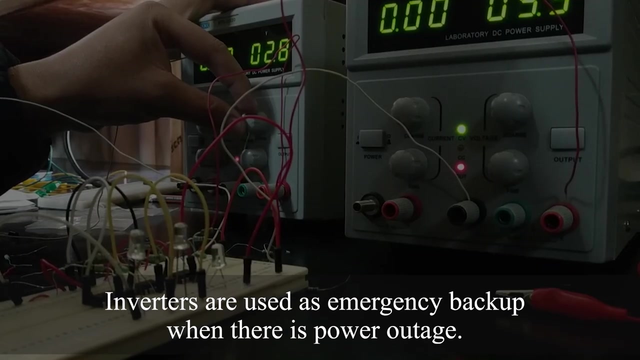 Let us check out this drone which can self-charge itself using solar power to increase its flight time. Let's see Rotating Solar Inverter. Project Inverters are used as an emergency backup. when there is a power outage, It turns on Electrical App. sadecerique ne222 KB resemble search module electricity. The 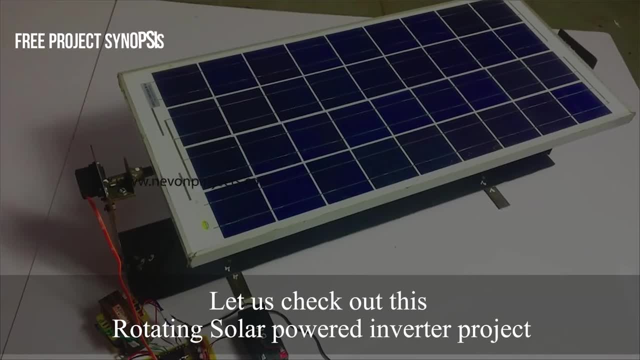 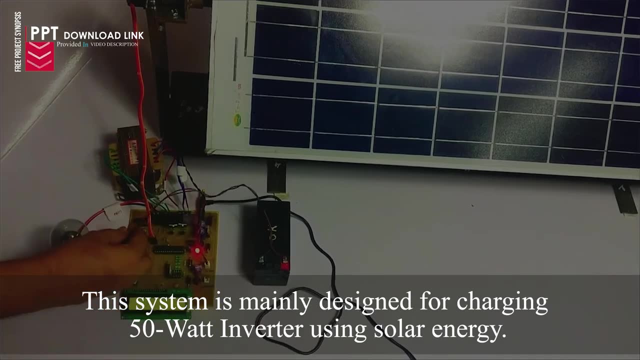 display on the far right reflects indication that the data collected by the printer Nestและ is when the main supply is off. let us check out this rotating solar powered inverter project. this system is mainly designed for charging 50 watt inverter using solar energy. 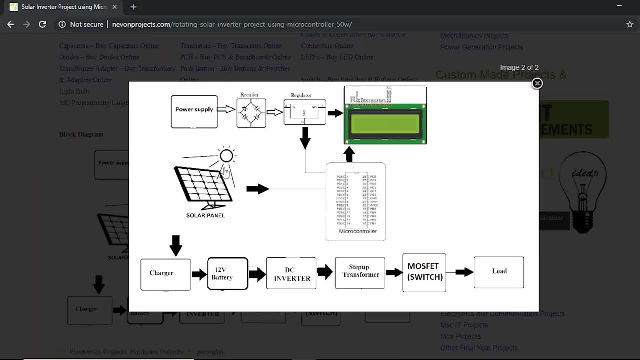 the server is used to position the solar panel at in the direction of the sun. how it does that is it checks for the voltage generated at each angle and the voltage which is the max voltage which is generated here. it checks the angle of that voltage and based on that it positions the 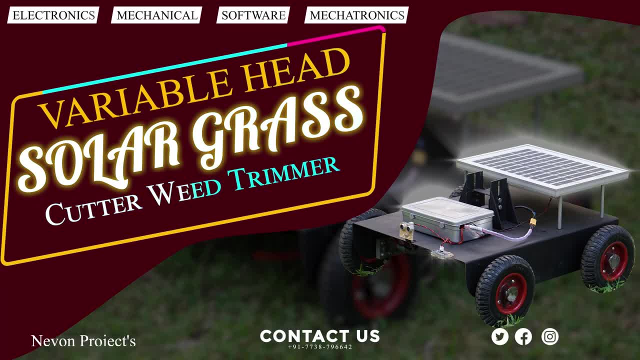 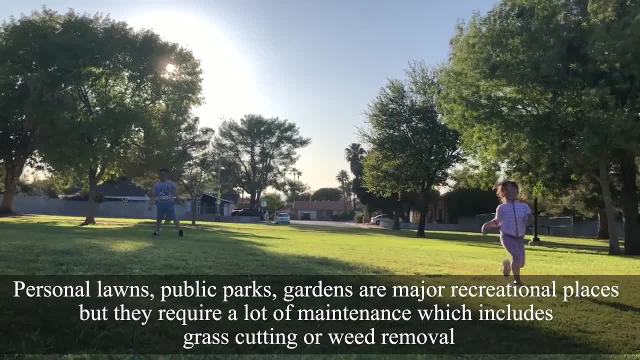 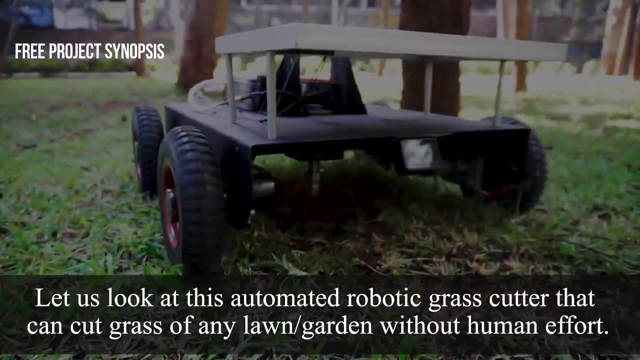 panel, variable head solar grass cutter. we trim a robot. personal lawns, public parks, gardens are major recreational places, but they require a lot of maintenance, which includes grass cutting or weed removal. let us look at this automated robotic grass cutter that can cut grass of any lawn or garden without human effort. 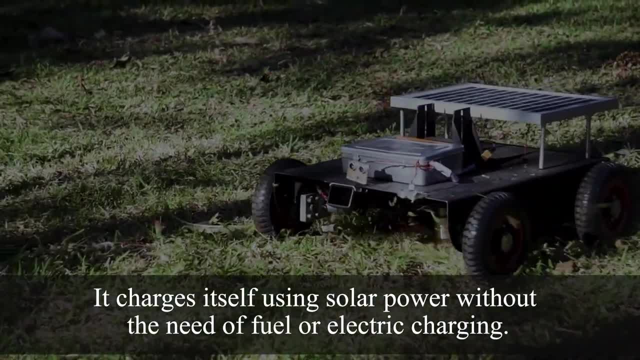 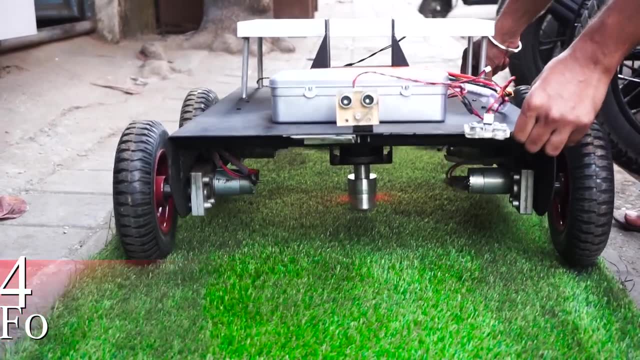 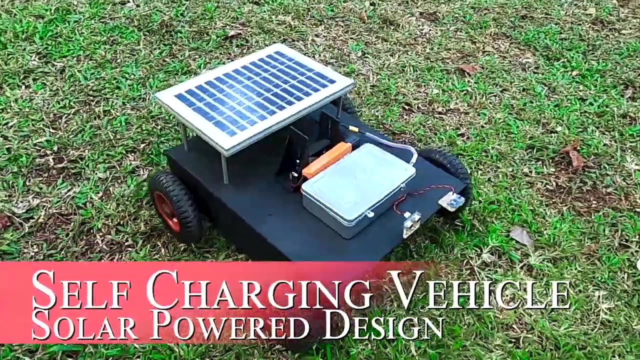 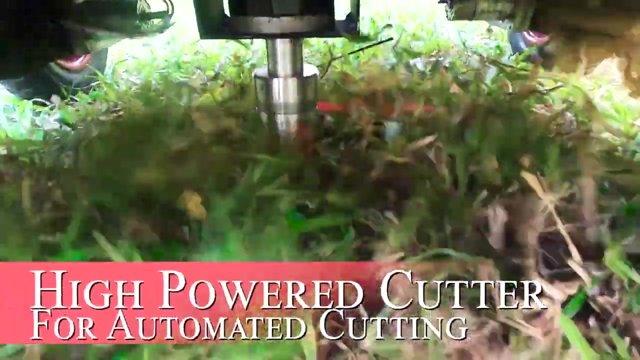 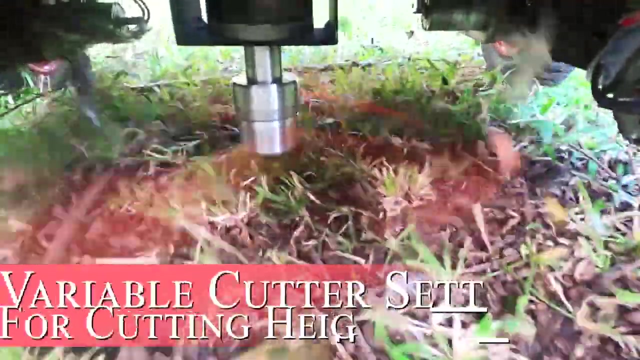 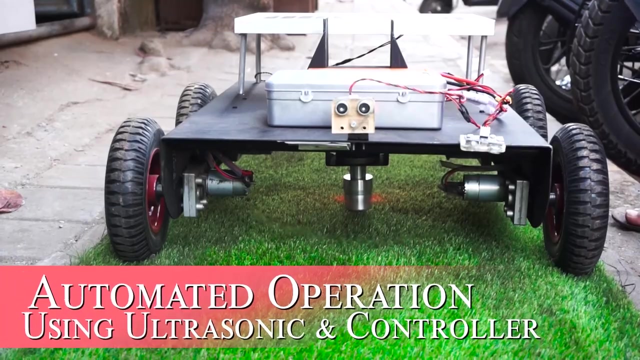 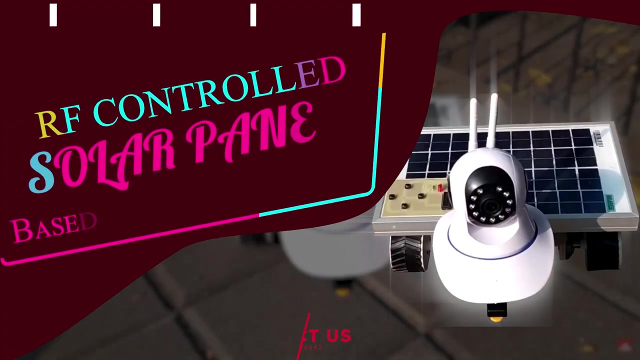 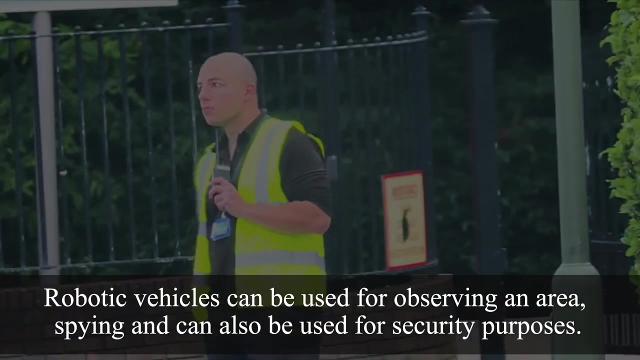 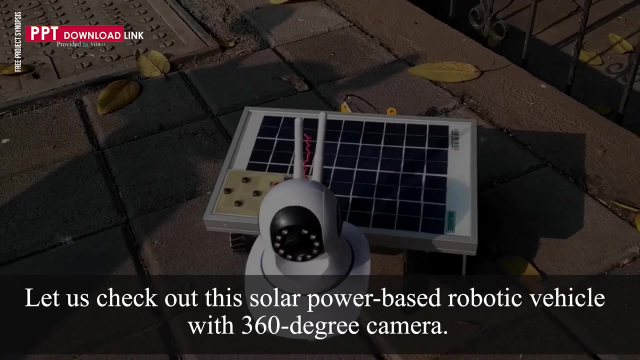 it charges itself using solar power without the need of fuel or electric charging. so rf control, solar panel based robotic vehicle. robotic vehicles can be used for observing an area, spying, and can also be used for security purposes. let us check out this solar powered robotic vehicle with 360 degree camera. 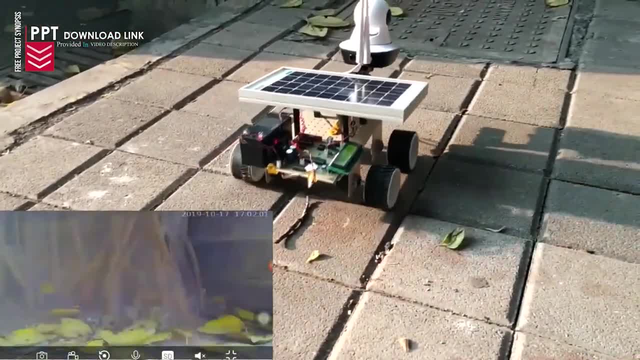 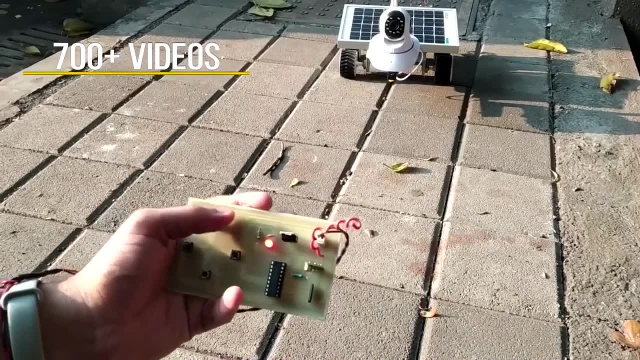 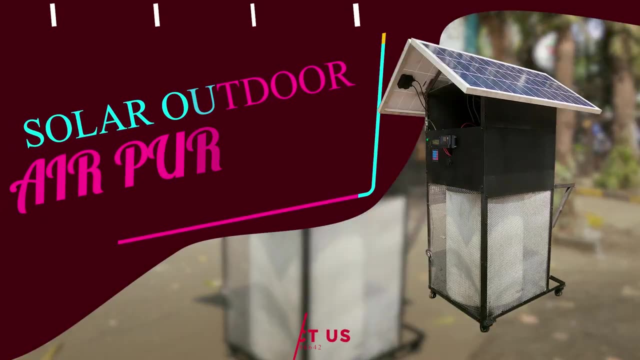 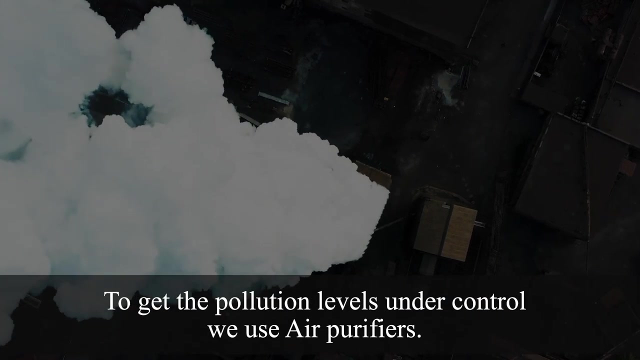 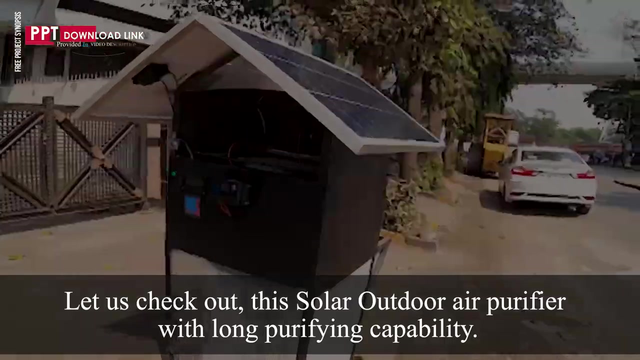 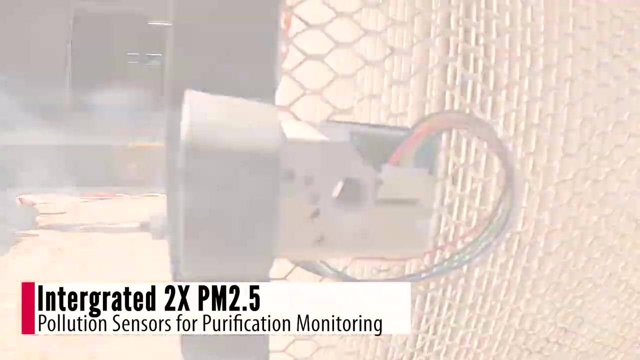 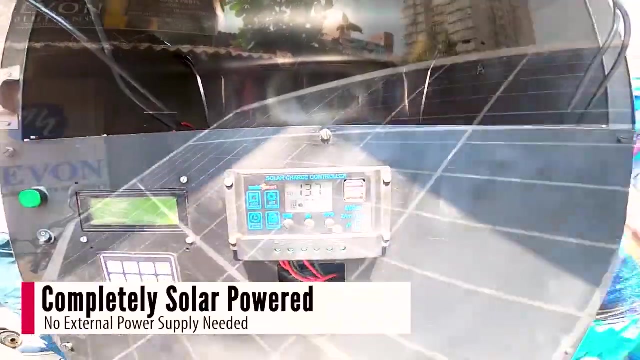 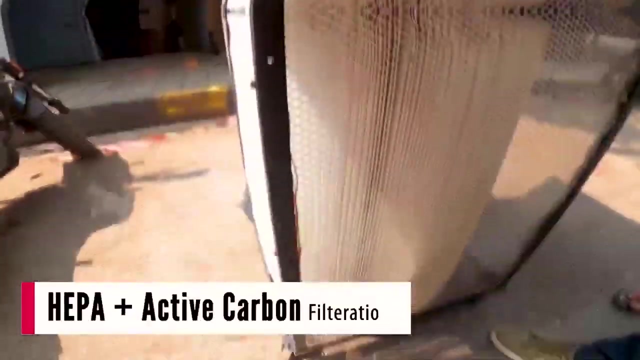 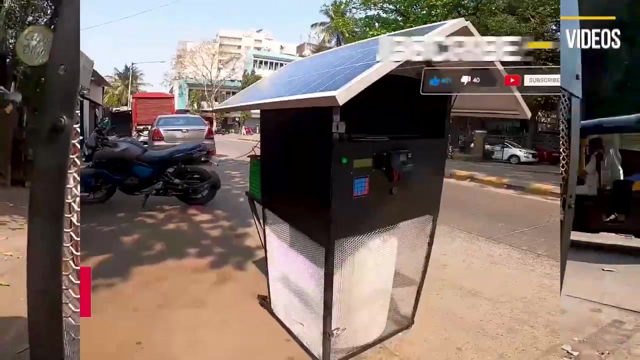 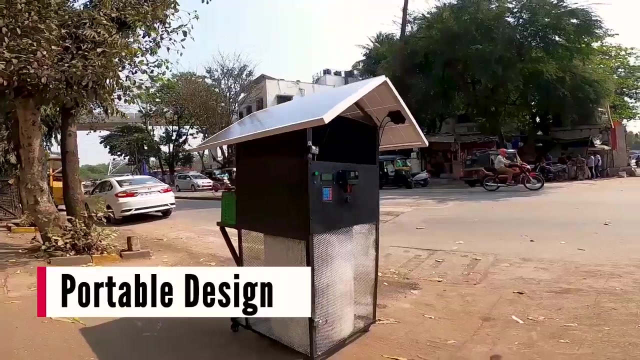 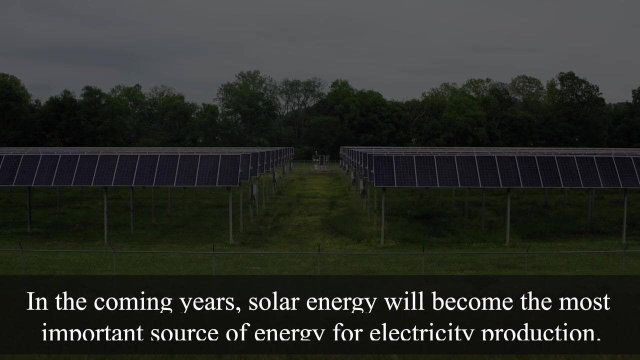 camera. Solar Outdoor Air Purifier. Air pollution is the leading environmental risk to health. To get the pollution levels under control, we use air purifiers. Let us check out this Solar Outdoor Air Purifier with long purifying capability, Dual-Axis Solar Tracking System with Weather Sensor. 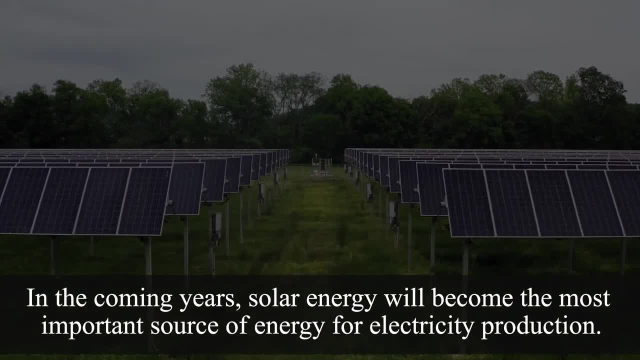 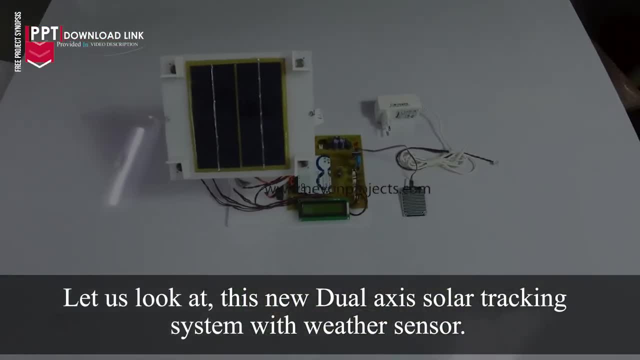 In the coming years, solar energy will become the most important source of energy for electricity production. Let us look at this new Dual-Axis Solar Tracking System with Weather Sensor. Solar Outdoor Air Purifier with Long Purifying Capacity. Dual-Axis Solar Tracking System with Weather Sensor.